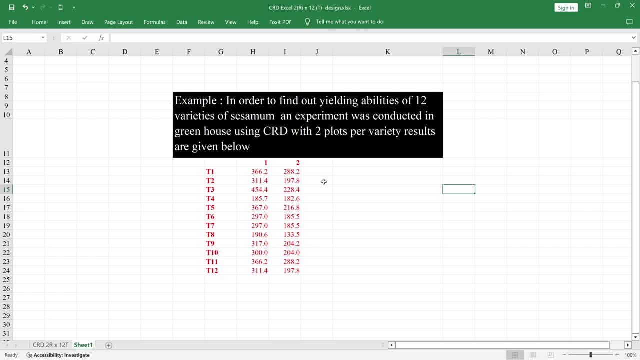 Hi, friends, in this session we will going to solve the example which is regarding the data analysis in Excel. We consider this experiment as a CRD design. You can see here the example. In that example we need to find out the yielding abilities of 12 varieties of 7 crop, and experiment was conducted in greenhouse. 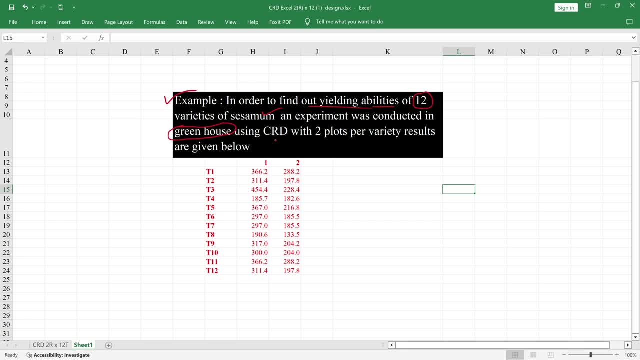 Keep in mind greenhouse, So that we consider the CRD design With two plots. If we consider two plots- oblique, two replications or two observations, all are equal, It's all equal. This means that if we consider two plots, then also we can consider two replications. If we consider two replications, then we consider two replications, And if we consider two plots, then also we consider the two replications, each variety You see here. Ok, So this is data given us for treatment: 12 and 1 and 2 plots. Ok, 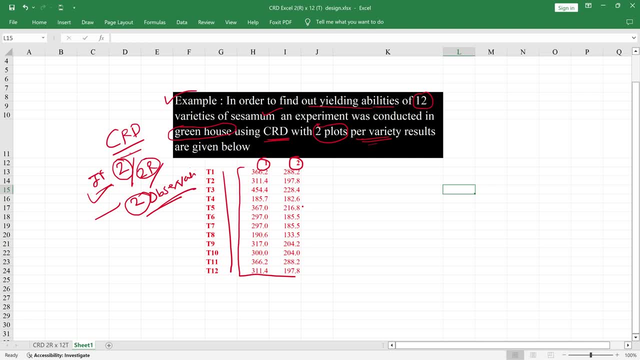 we need to do the analysis of this data. it's very simple. we developed so many excel designs for the different treatments and different replications. if you want this type of excel sheet for your data analysis, then definitely you contact us. you just need to copy this data. okay, you can copy this. 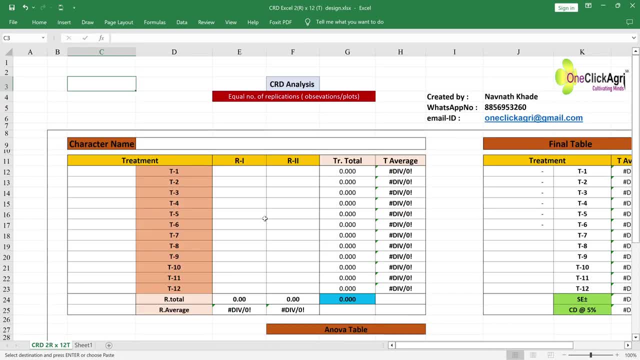 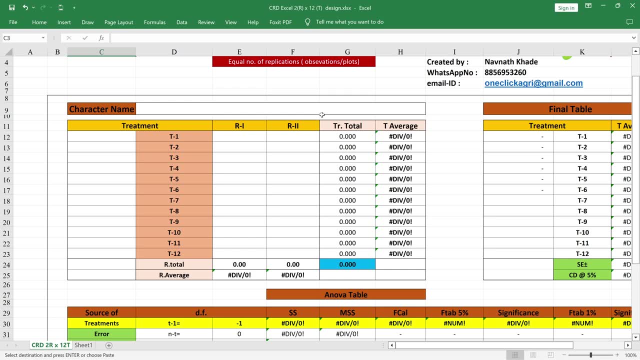 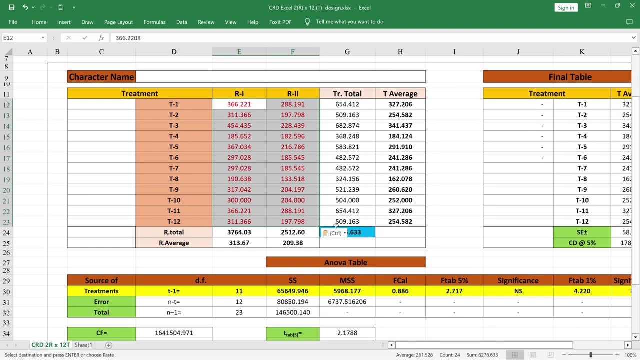 data. and come to our excel software. okay, this software is for equal number of replications or observations, or plot. okay, what you need to do only here, you just click here, right click and paste the data. okay, everything is fully automatic in this. then you will get the grand total. then. 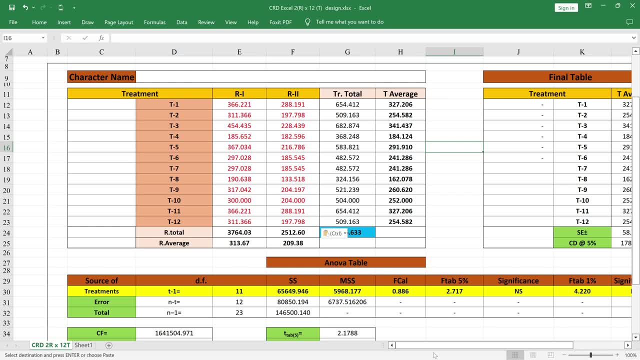 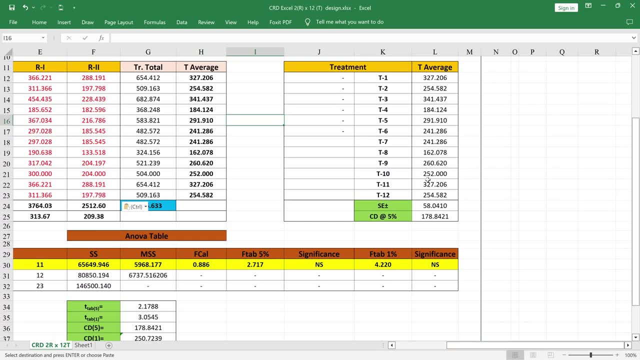 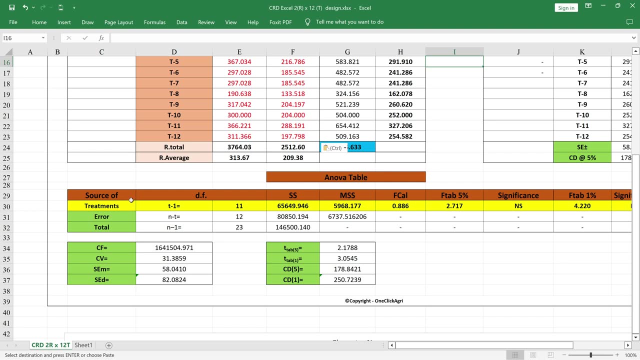 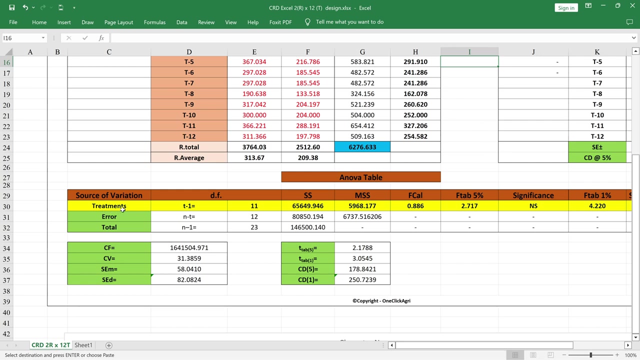 replication mean, then treatment mean you will get here. okay, so you will get the final ANOVA table, final thesis table. you can see here the final ANOVA table. you will get the source of variation. so in source of variation you will get only the treatments right. why? because this is crd design. 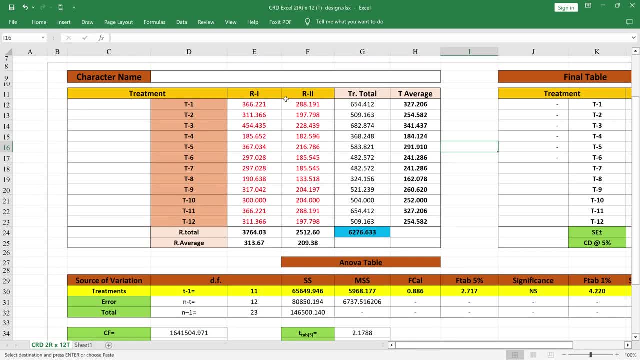 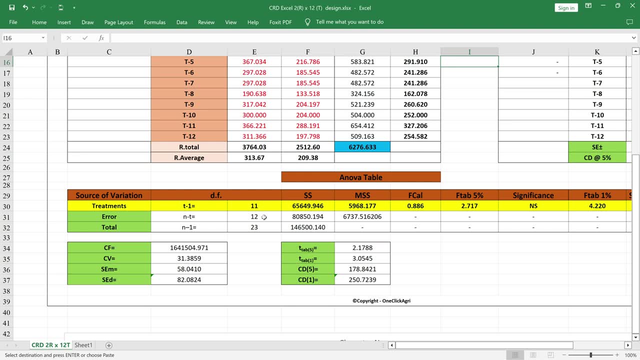 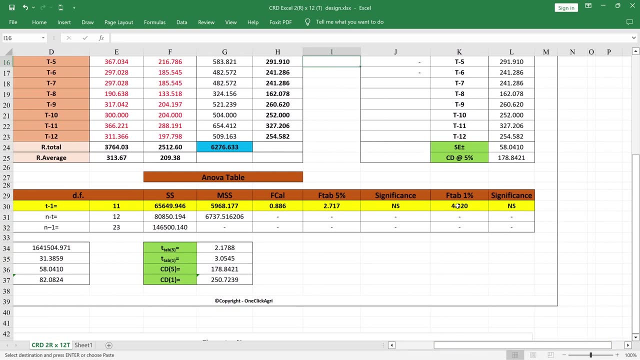 we don't consider the replications over here, just we put the observations over here. so we consider the source of variation only that treatments you will get the degrees of freedom. sum of square means sum of square, then f calculated, f table significance and these statements are non-significant. 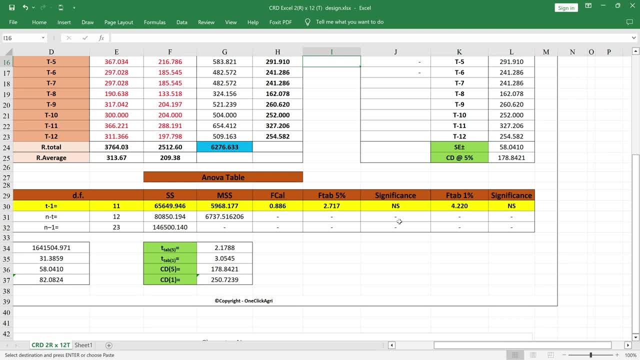 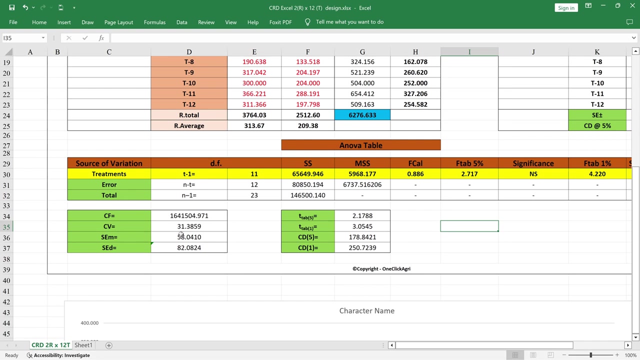 if statements are non-significant, they not need to calculate the cd value and further analysis for this. okay, because if there is no difference among the treatments, then no point to calculate each treatment. if it's because all treatments having same effect or same yield, then you'll get the main value here, the cv value, and this cv value is too high. 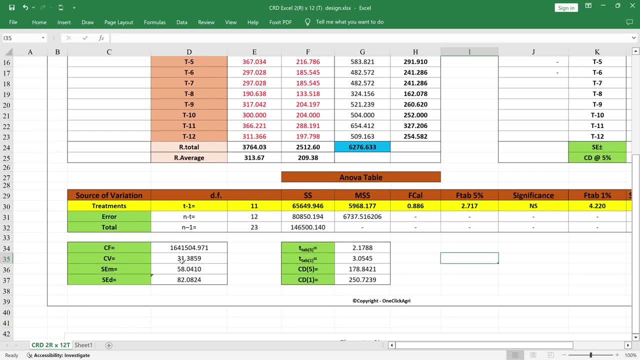 that's why it's showing non-significant. okay, because in crd design, we should have to consider the cv value below five percent. okay, keep in mind this is, you know, this is the very high. okay, so for crd design we need less than five percent. okay, keep in mind this. 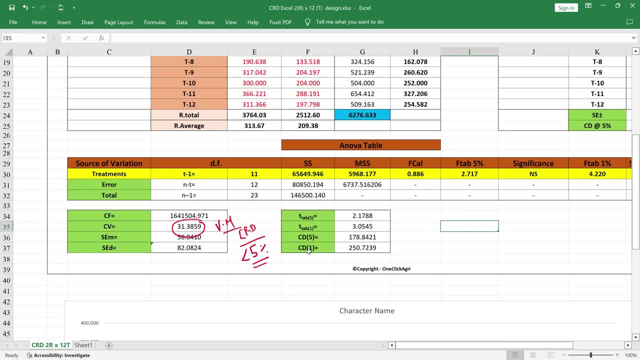 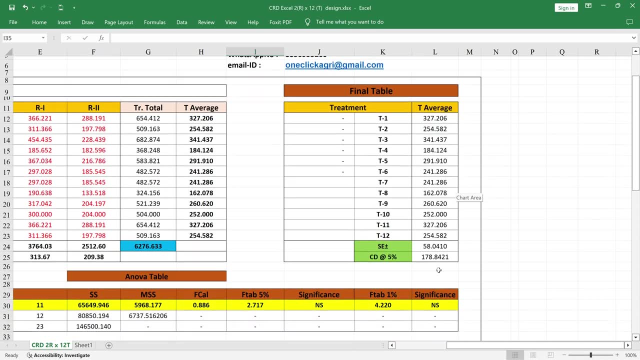 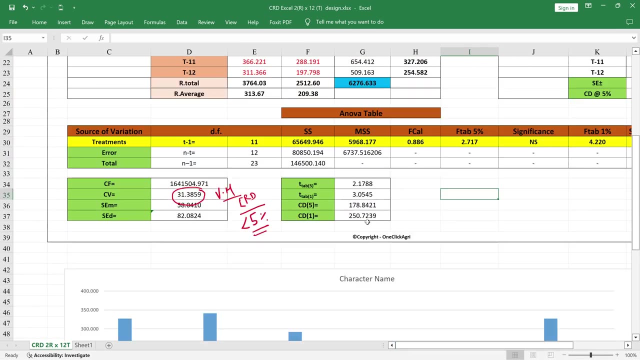 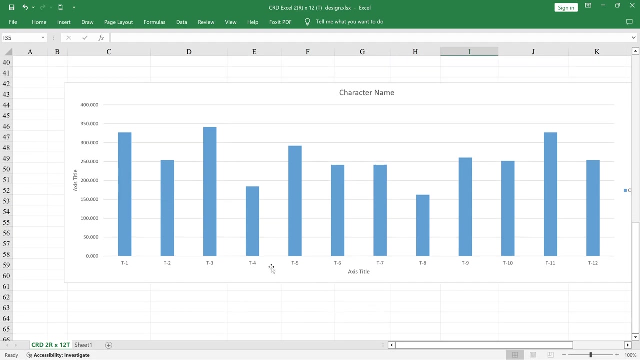 in another one you will get the cd value for five percent and cd value for one percent and this is the final your thesis table. you can copy this table and paste you in your thesis. then below you will get the graphical data analysis. in that you need to only edit your.